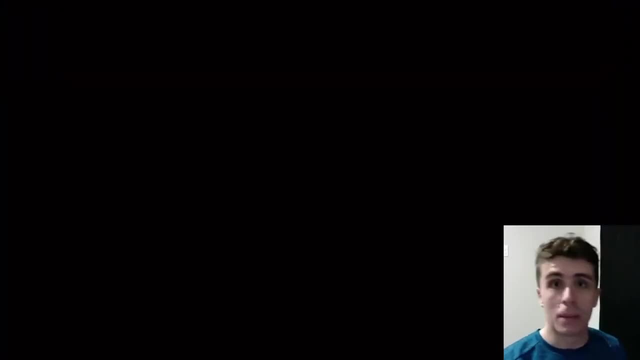 of a parse tree video I did a while ago. So today we're going to be talking about parse trees for context, tree grammars and leftmost derivations. So here you can see me rattling on about some random nonsense. blah, blah, blah. parse trees, yay. So I think I'm going to. 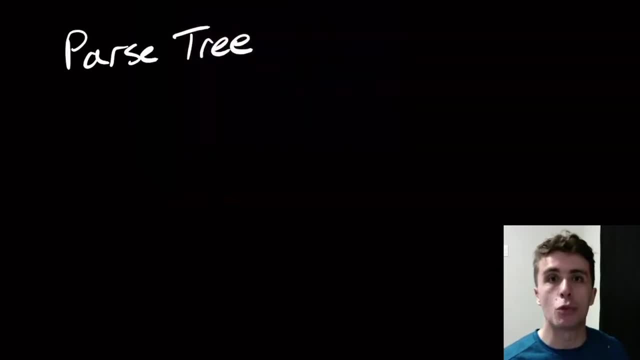 talk about. so I don't have my script in front of me because I never have a script, but so I'm talking about parse trees for a long time. We're talking about a context tree grammar and maybe we'll talk about, like, the structure of all of the derivations in them. Yeah, so parse. 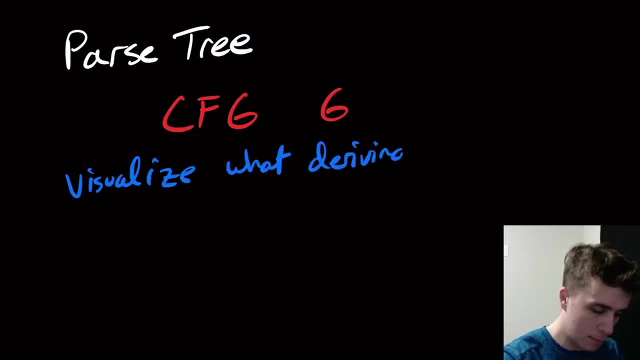 trees are a visualization of what a derivation looks like When we derive a string by applying rules over and over and over. it's just a visual representation of what that process actually is. All right, so I look quite confused in the things that I'm saying. but yeah, so let's see. 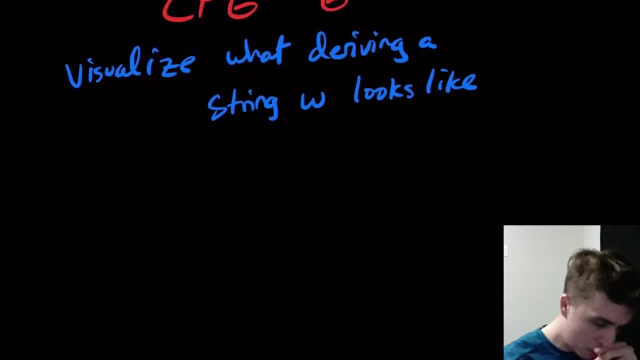 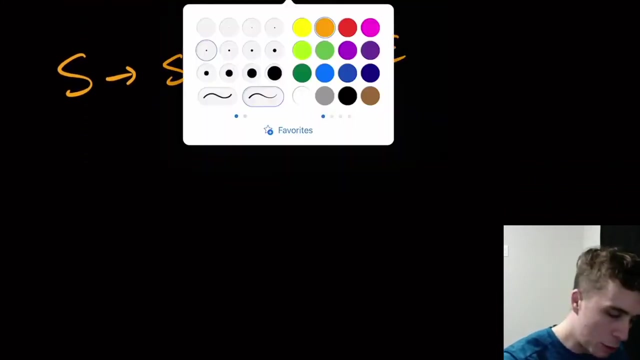 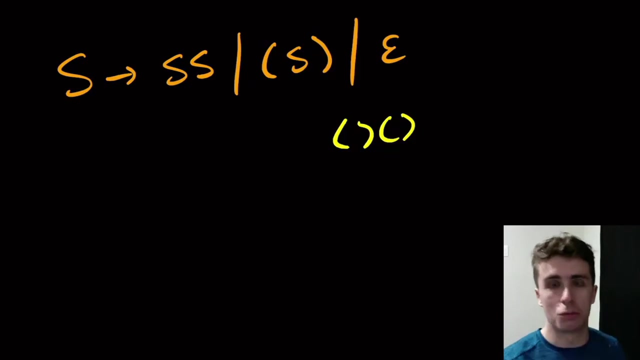 what am I going to say next? What is Ryan gonna say next? All right, so here I'm guess I'm doing left s right, or epsilon, so that's the set of balanced parentheses, or the grammar for it at least, And here I'm trying to derive the string left right, left right, so that's a set of balanced. 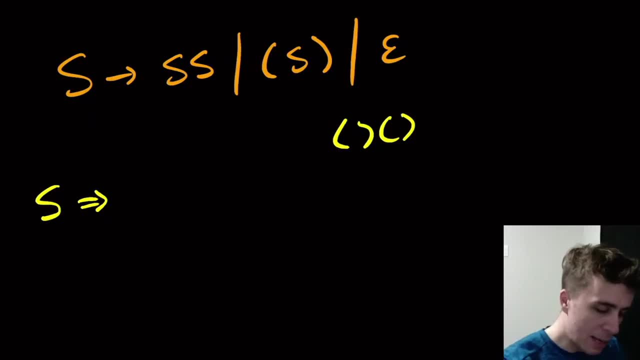 parentheses and it's easily derivable in this grammar in the way you have to do the ss rule here. So s so I have to apply. it goes to ss here. and then here I have a choice. It's of whether I can apply the left s right to the first one or to the second one. So here I do the. 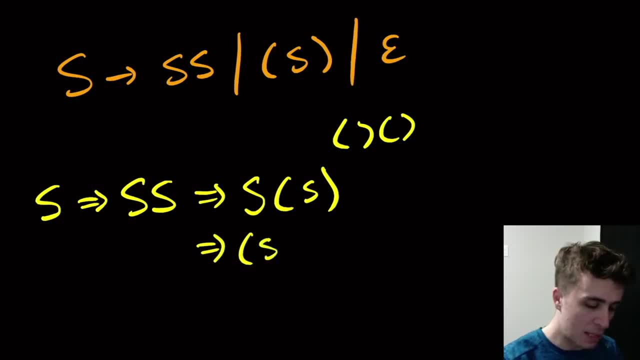 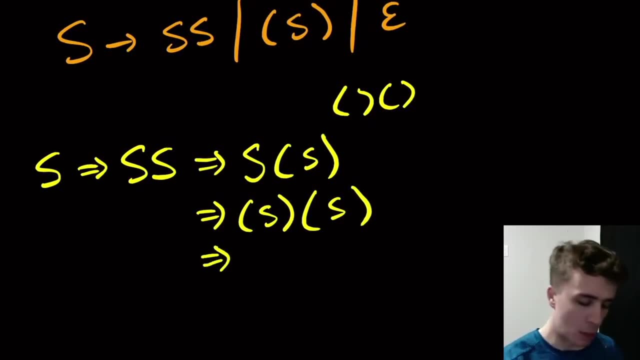 first one. Sorry, oh my god, second one, And then I do the second one, and then I'll make the one of the two s's go away. I think I do the second one. yeah, So I make the second one s go to empty and 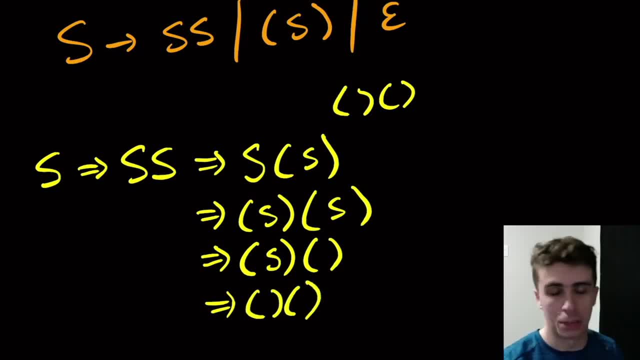 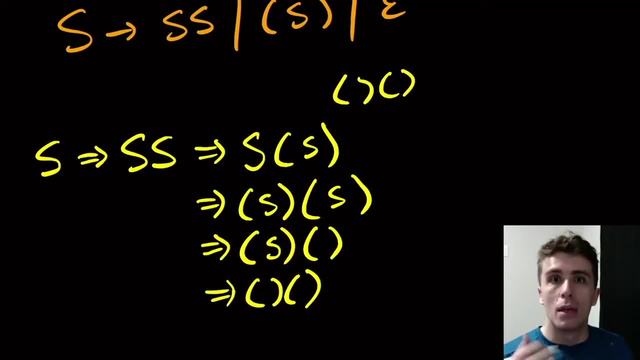 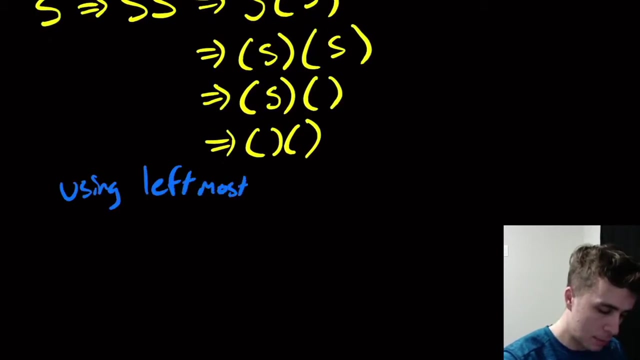 the other one and the first one go to empty. Yeah, so that's one way to derive the string, And I think all what I'm gonna do is I'm gonna show another way to actually make the string- the same string in the same grammar- And what I'll probably do is I will let's see. okay, yeah, so. 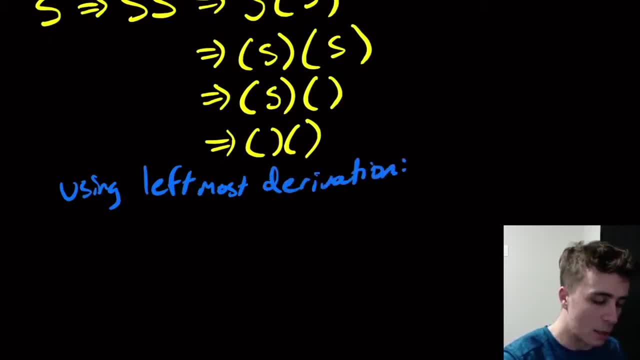 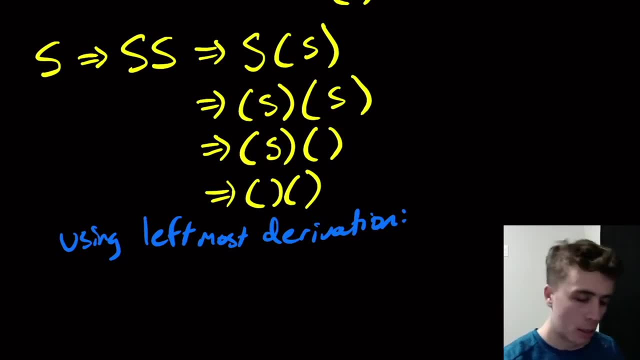 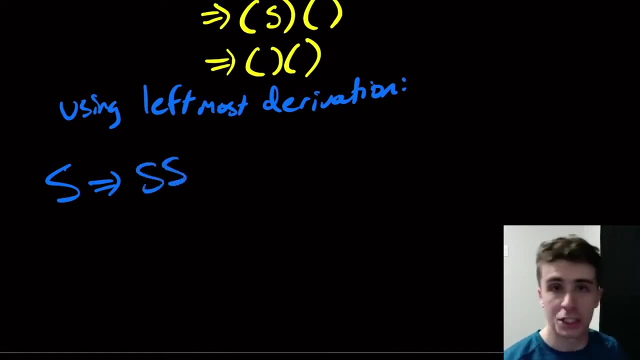 notice that I could have chosen the left or the right s up there. I didn't there was. I pretty much had a full choice there. But using something called a left s, right s, I could have chosen the leftmost derivation. I always will choose the leftmost variable in the derivation. so far I 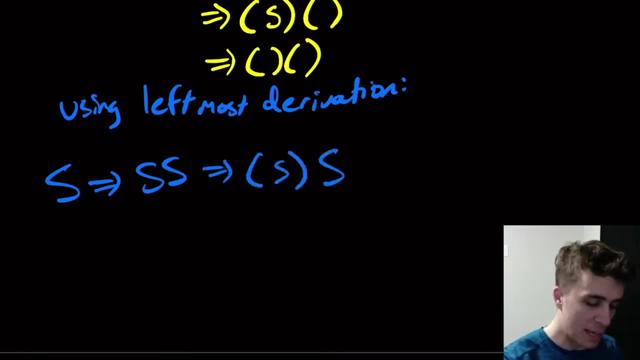 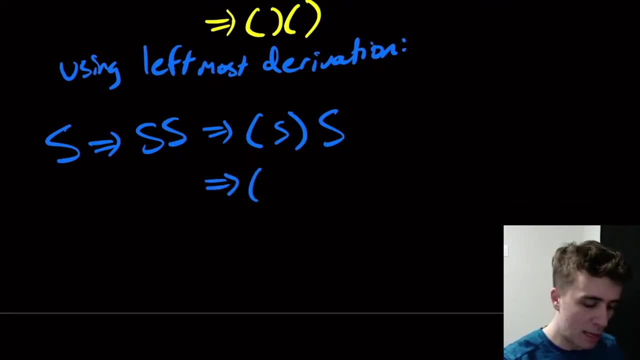 will never choose a different variable. So here I replace the first s now, and then I'll replace that first s yet again with empty, And then now, since there's only one variable, then I'm going to work with it because it's the leftmost one, and then make left s right and then have it go to empty again. 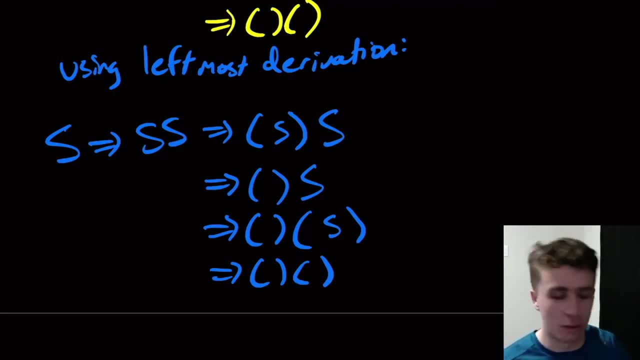 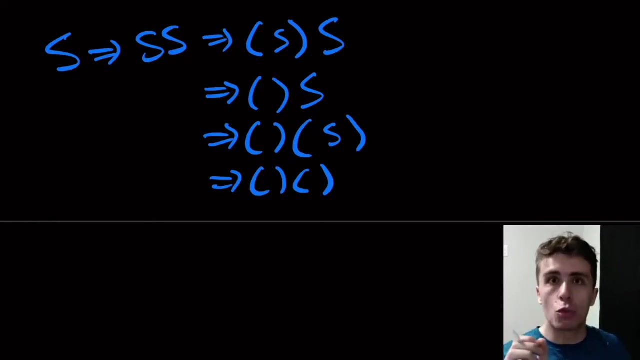 Alright. so I think what I'm saying here is that in, in any derivation I can always use, I can always find a leftmost one, because there's always a leftmost variable, And so I can always work with it because it's a context-free grammar. It doesn't matter what the context in which the variable is. 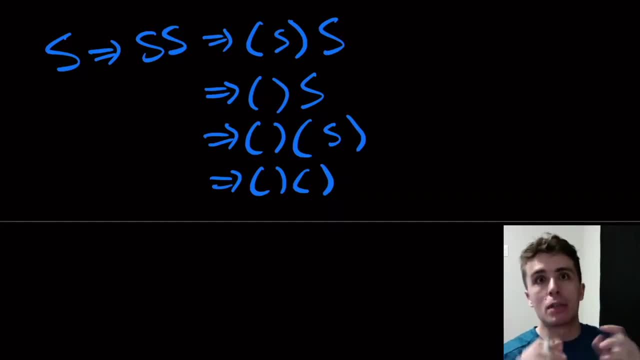 So I can. I can work with it completely freely of all the other variables, So I might as well just choose the leftmost one, Okay, so then now I'm here, looks like I'm talking about what a parse tree is, So it's a visual. 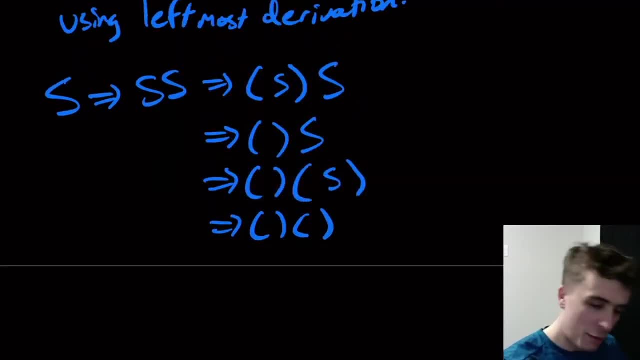 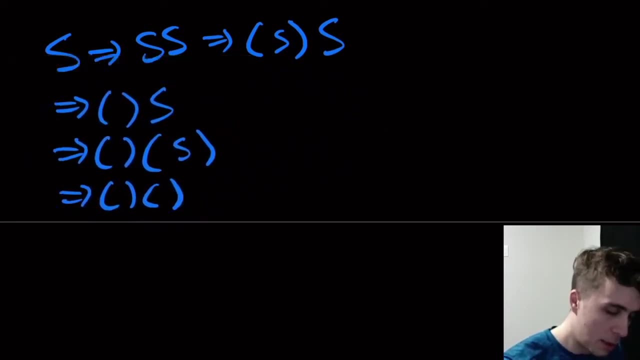 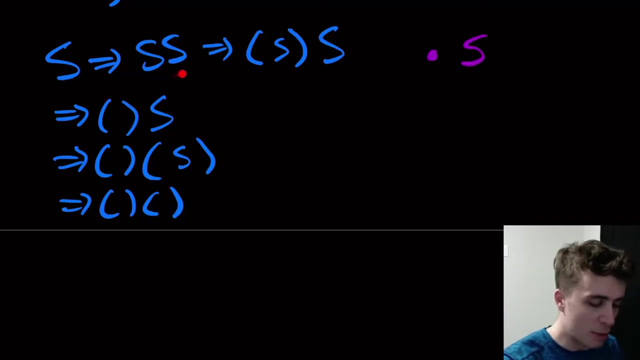 representation of what this looks like. So a tree in computer science is you have a bunch of nodes and all of the nodes underneath a node are the children of that node, And a parse tree has elements of variables or terminals, as the nodes and the ones that have children are the variables. 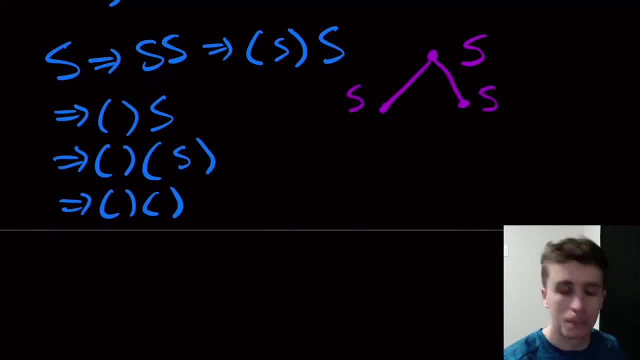 themselves S up top is the first s. The two underneath it are the two s's. So s produces ss, is that first s up top makes the two s's down beneath it. And then now we will look at the left s, the one I'm circling. 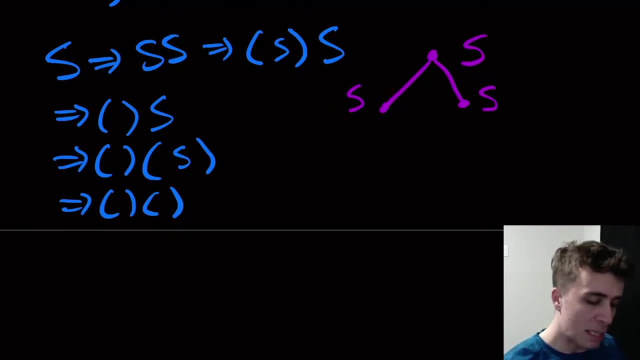 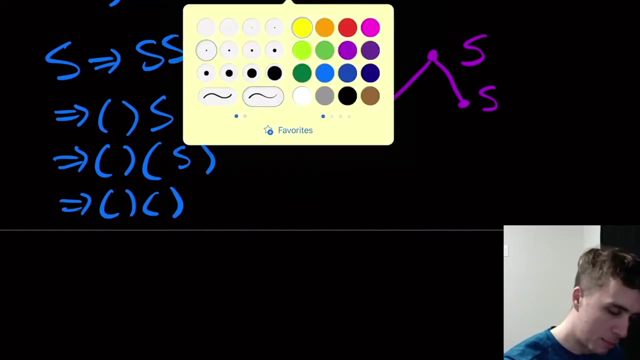 now and then. the right s there, The left s is going to make the left s right, So that one's going to have three children, which are the lefts. Oh, it looks like I do different colors here. Make the left s right. 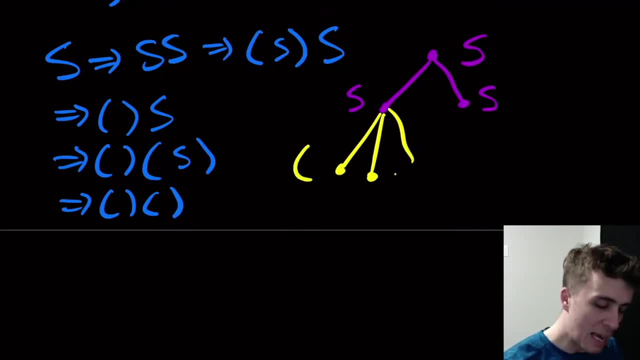 Make it pretty. So then I have left, and then the middle one's going to be s, and then the right one is going to be right, And then the, and then it's going to look the same on the other side because it's symmetric, But the middle s is going to produce empty because we- we chose that rule for. 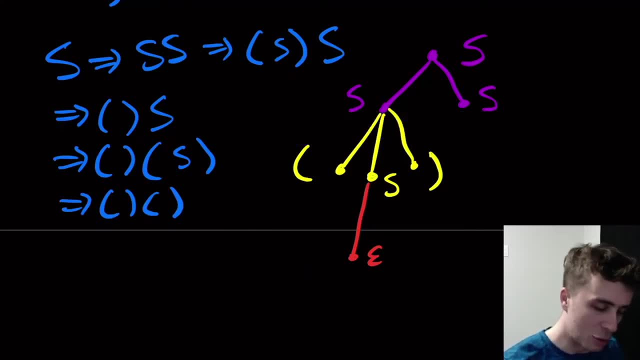 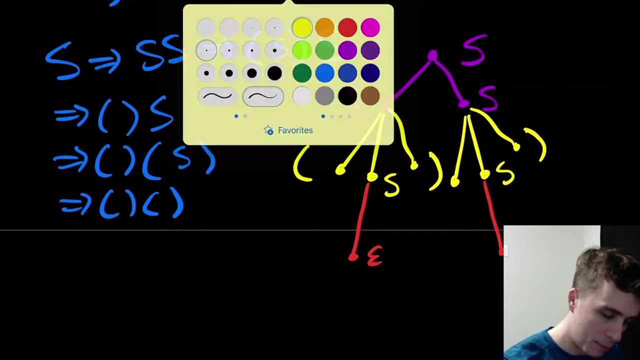 that variable s. So here it looks like I'm going to copy and paste it over onto the other side because it's completely symmetric And it looks like I'm going to have trouble Trouble fitting it all on without colliding. It's one of the issues of having a really small screen to depict a lot of info. 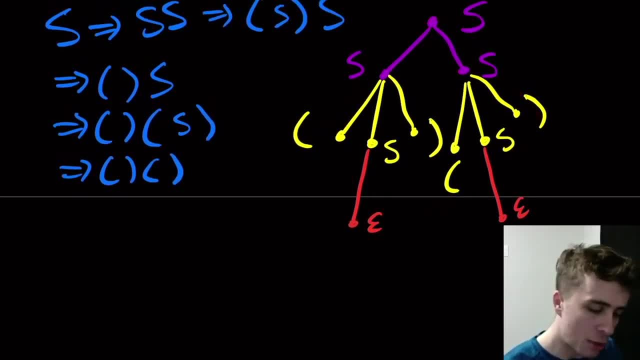 So that's what a parse tree is, or an example for this particular grammar. All right, So what am I rattling on about now? And so the way to figure out what the the, the parse tree, actually corresponds to is, do you write it in a way that it's not a? 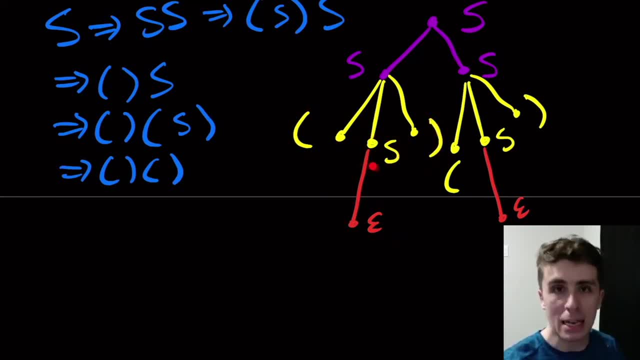 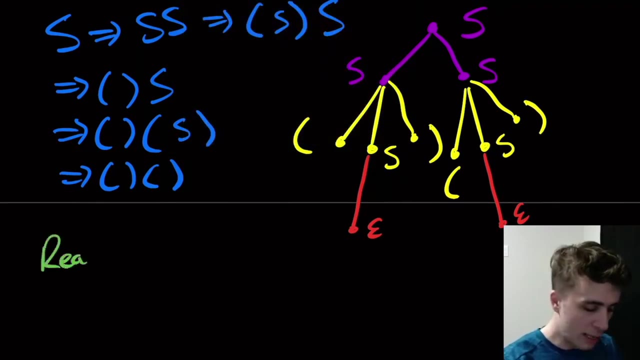 read the terminals which are at the very bottom of the tree, all of the leaves from left to right. so if you read them from left to right you will have left empty right, left empty right and there are certain tree traversal algorithms to find out what those are. but here I'm saying, if we just read the leaves from, 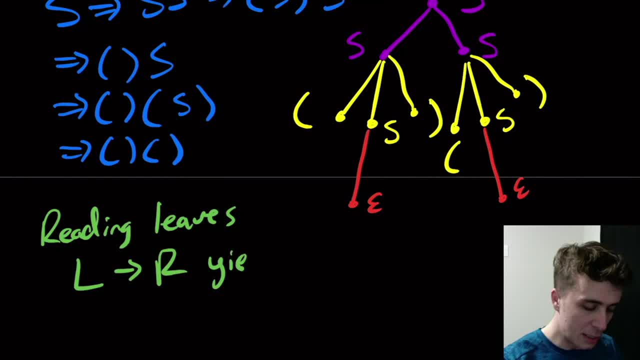 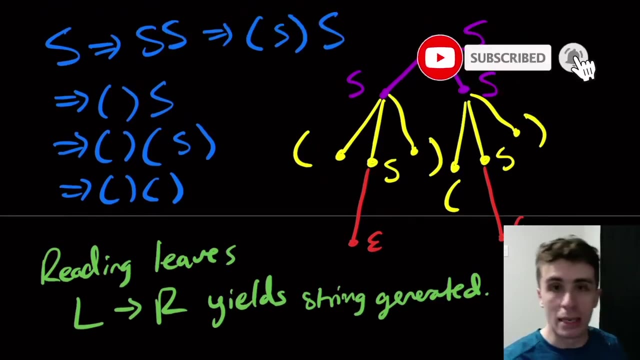 left to right, then that's the string that the original derivation produces, which is exactly what we want. so one thing that you can prove is that, left, most derivations correspond exactly to parse trees. yes, please subscribe, subscribe, please click the bell too. please click the bell so you get all. 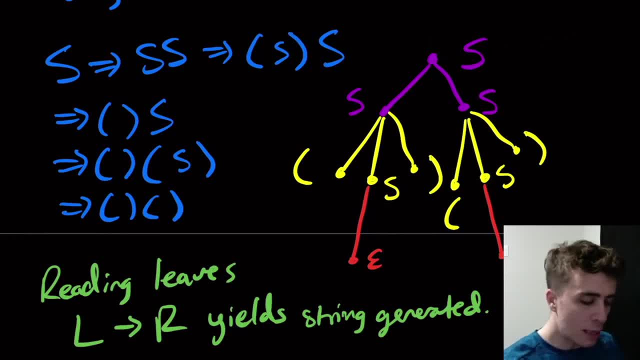 notifications of easy theory stuff. let's see what else am I gonna say here. so I'm circling a variable. why am I circling a variables? so it produces those children. yeah, we already know that silly. okay, whole parse tree. there's the whole parse tree and the derivation. so here,